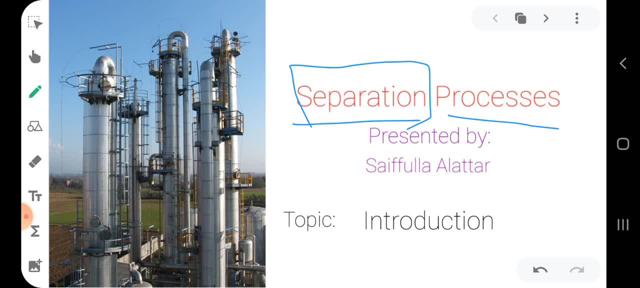 components or more so at least. we need to have two components or more, three, four, five, and we want to separate these components from one to other to some degree. we cannot split perfectly, but we need to split to some degree. okay, and we need to separate our interested product from the others. and to start with, let's discuss different type of 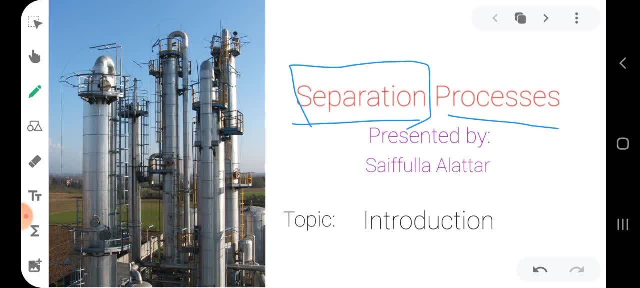 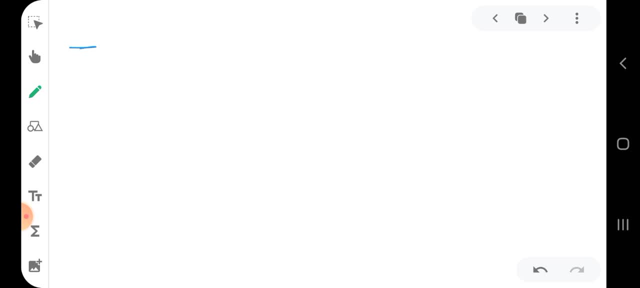 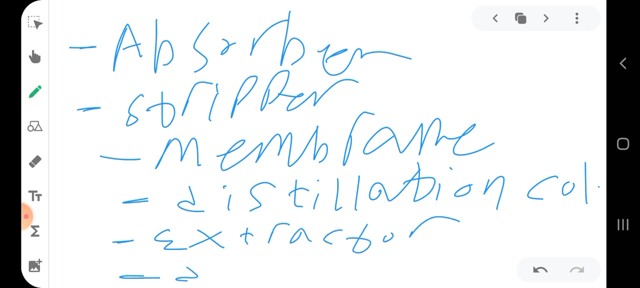 separators that we may deal in chemical engineering first and we have two. we have too many different units and chemical engineering related to separation process, like the absorber, the absorber and stripper and membrane and distillation, distillation column and extractor and dryer and adsorber, etc. 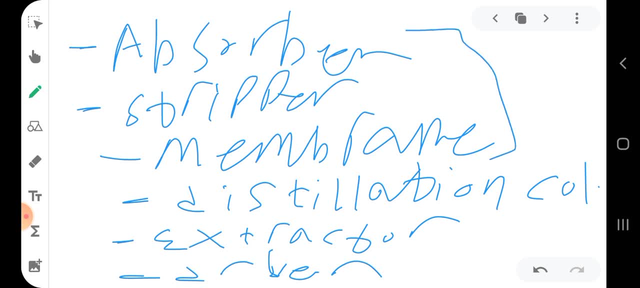 the first three absorbers- stripper membrane- you may discuss- and the mass transfer course. in this course we are going to discuss the other types, like the distillation column, the extractor and the dryer. the main difference between this course and your previous mass transfer course is that in 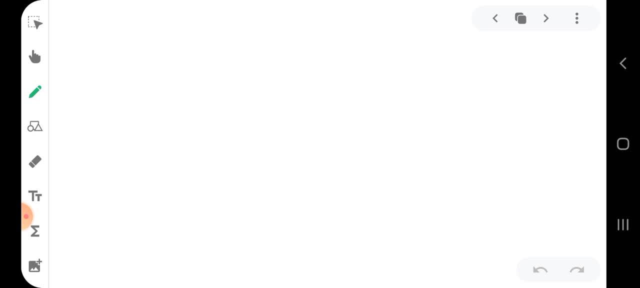 analyzing separators. we have two different models, so we have different models to analyze the separators. first is called the rate based models and the second one is called the equilibrium based model. what's the main difference? the rate based models, which you have discussed in your mass transfer course, as it's like when you say that any flow is equal to a mass transfer. 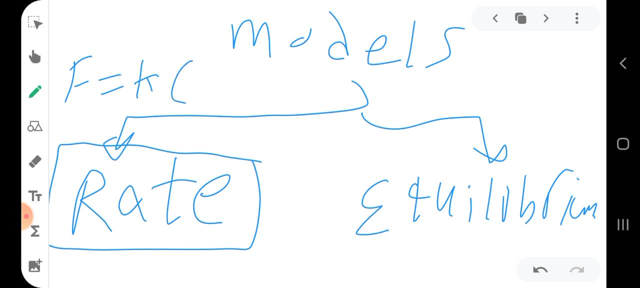 coefficient times the driving force, which may be at the concentration difference for the mass transfer. okay, so it's based on the rate and we are using a mass transfer coefficient which is k or f if you have a concentrated solution. anyway, it's a mass transfer coefficient, okay, so it's like we have a driving force and we multiply. 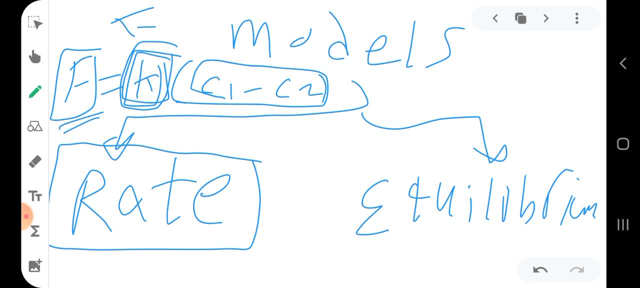 it by the mass transfer coefficient to get the flow. okay, this is the rate based model which you have discussed in the mass transfer course. now, in this course, we are going to discuss another type of models, which is called the equilibrium based models. what do we mean by? 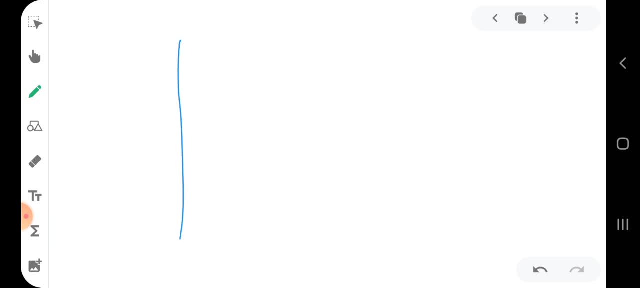 equilibrium based models. these models are based on having a data for the equilibrium. it is like when you have a two-way system: so this is the liquid and this is the vapor, and let's say you have two components, maybe component a and component b. they are in the 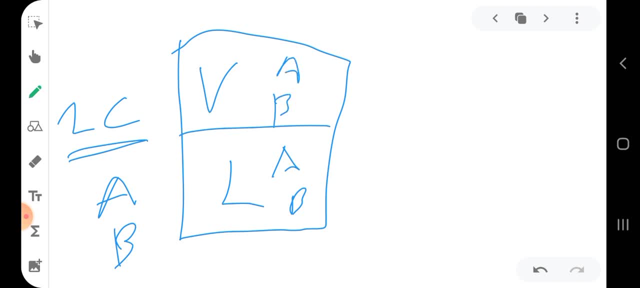 liquid phase and they are in the vapor phase. and let's say the concentration in the liquid phase is the vapor phase is y. so to use the, the equilibrium based model, first you need to have a data for the equilibrium. what's the concentration and what's the more fractions and the v in the liquid phase? 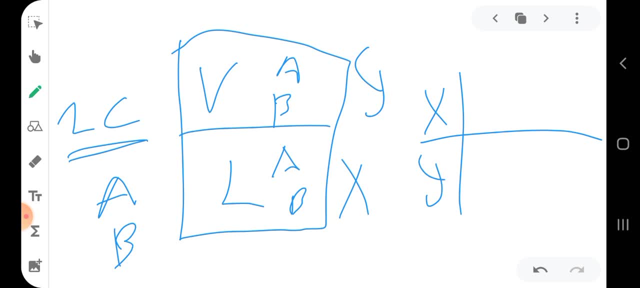 and what's the corresponding more fraction in the vapor phase. so you need to have this data before starting using the equilibrium based models, okay, or any information from where you can construct this table and then you can start your solution. this is the equilibrium based models. okay, now let's talk about the other, about the other. 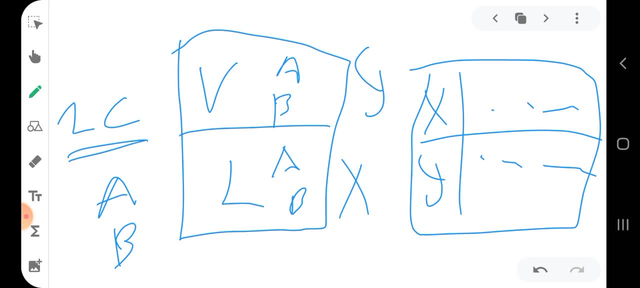 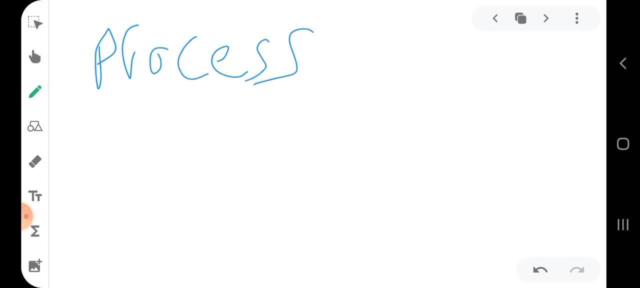 one and the title? the title was separation processes. so what do we mean by process? what's a process? a process is something that accomplish another thing. that's a simple definition of the process, and we have many different types of processes. first, based on the time, we can have steady state process and we can have unsteady state. 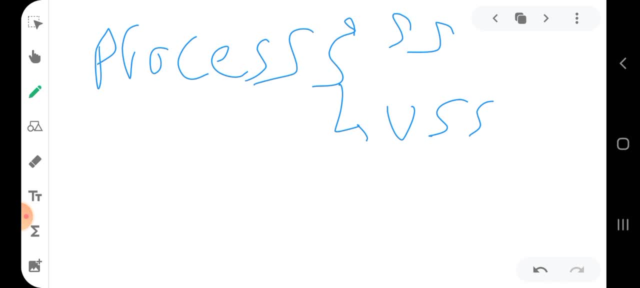 process of transient process and steady state or transit are the same ones. uh, so these models are this: based on the time, we can have steady state forces and an unsteady state force. in the steady state process, there is no change with time and in the unsteady state process, the process change with. 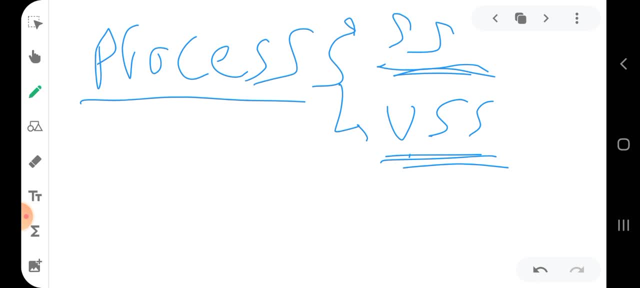 time. so this is based on the time and based on the streams. we may have a batch process or semi-batch process or continuous process. in the batch process, there is no feed and there is no products. in the semi-batch process, we may have only feeds with no products or only products with 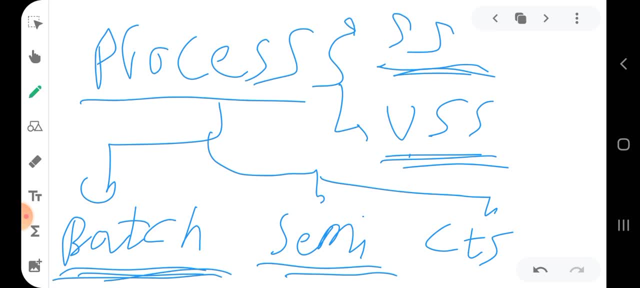 no feeds. in other words, we may have only inlets without outlet, or we may have only outlets without continuous inlet, and in the continuous process we have a continuous inlet and outlet from any unit. okay, so this is introduction, based on the title. now let's discuss. what are the 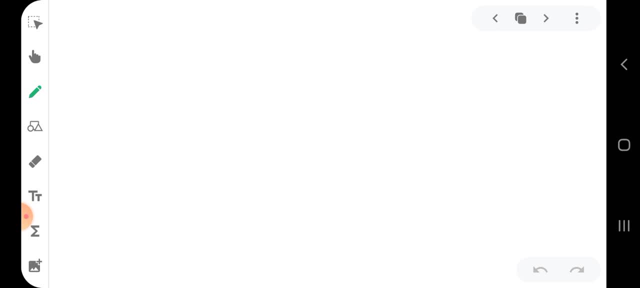 main courses that we need, the previous courses that we need in this course. first, we need the material balance course. we need the material balance course. what do we need from this course? we need to know how to do a material balance on single units, multiple units, but without reaction. i'm not interested. 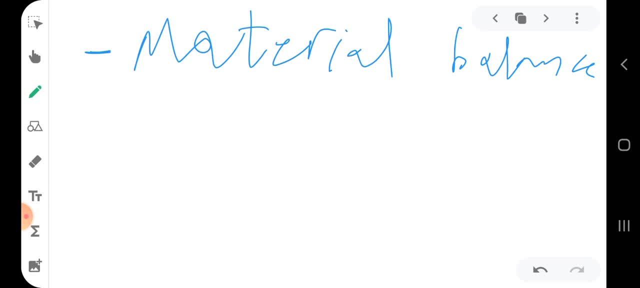 on chemical reactions in this course. okay. and also, what do we need from thermodynamics conditions? we need the capacity relax soil, then we need the bond sealing. that what we need. and theе equilibrium. which equilibrium? as you know, we have two types of equilibrium in chemical engineering, which is the chemical reaction equilibrium and the base equilibrium. mainly of we need only the base equilibrium, not the chemical these equilibrium, which you may discuss in your chemical reactor design course. in this course separation process, we need only the phase equilibrium, not the chemical reaction equilibrium, which you may discuss in your chemical reactor design course. in the Ant residential 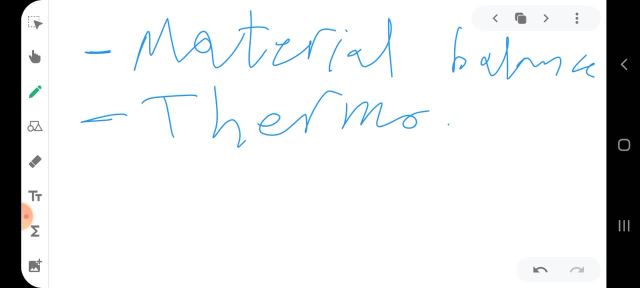 cost separation, the solution process, this course separation process. we need only the vase equilibrium, where you have two vase system, like, for example, liquid and vapor, and you need some equilibrium relations to to deal with. okay, so that's what we need from the thermodynamics course and from the computer application course. 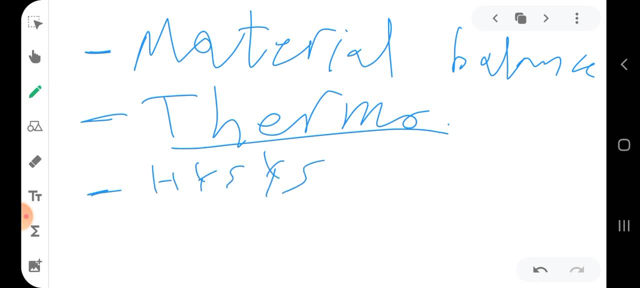 we need to know how to use ISS to simulate, to simulate some separation processes and from the numerical cause, from the numerical course, uh, we need, uh we are heavily depend on the graphical solutions, which is an approximate solution. we are going to deal a lot with the graphical solution. 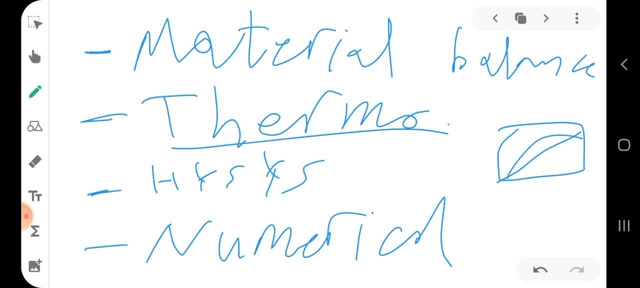 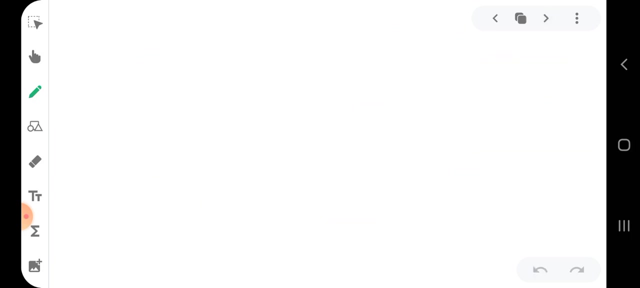 whether you need to graph and then solve the problem. okay, so that we need from the numerical course also, we need to know how to use the numerical integration to solve some problems, as we will see in this course. okay, now i'm going to discuss what we are going to discuss in this course. 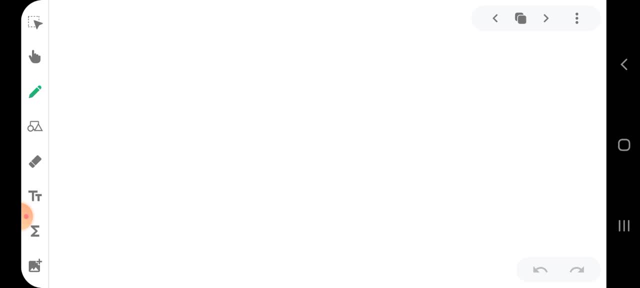 okay, in this course we are mainly going to talk about three, three units of separation only, which are that distillation column- we are going to discuss the distillation column- and the extractor and the dryer, but mainly we are going to discuss the separation of the two units. 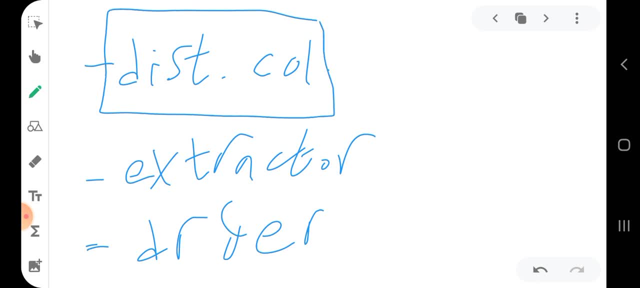 going to focus on the distillation- this is our focus- and then we are going to discuss the extractor and a little bit of the drying process and and in analyzing the distillation column, we are going to discuss two types of operating modes, which are the steady state and the unsteady state. 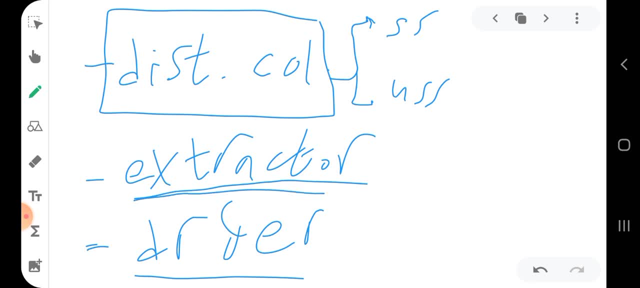 okay, and in analyzing the extractor, we are going to discuss only the steady state process. dryers: we are going to discuss the steady state process mainly, and the unsteady state will be discussed as a theory part. okay, and for the distillation? for the distillation either, 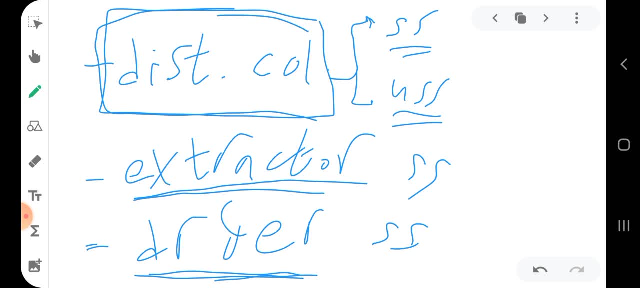 the steady state process and unsteady state process are going to be clustered together in definition. stage state process, we are going to discuss two different types of columns, okay, which is the single, the single stage distillation and the multi-stage distillation. again, in the extraction process, we are going to discuss same: the multi and single stage. 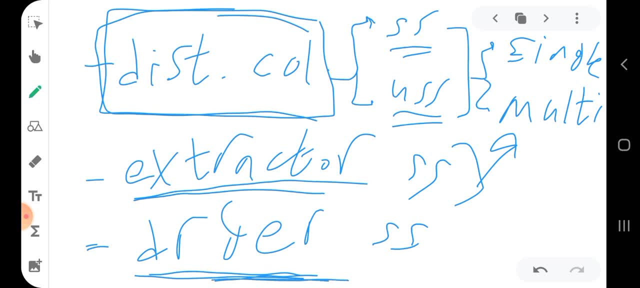 processes and in the dryers. i'm not going to discuss these types. we will discuss other types, as you will see later. okay, but an important question is: what do we mean by single stage distillation and multi-stage distillation, or single stage process in general and multi-stage process in general? what do we mean by a stage? 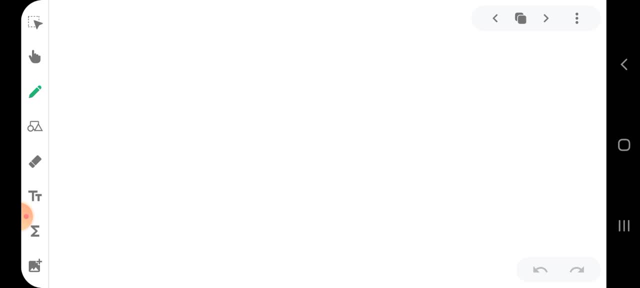 what do you mean by a stage itself? a stage is a place where the liquid and vapor or gas meet each other, and we are going to assume that the equilibrium is reached in this system, and a stage could be a plate or anything that where the liquid and gas or vapor met each other.